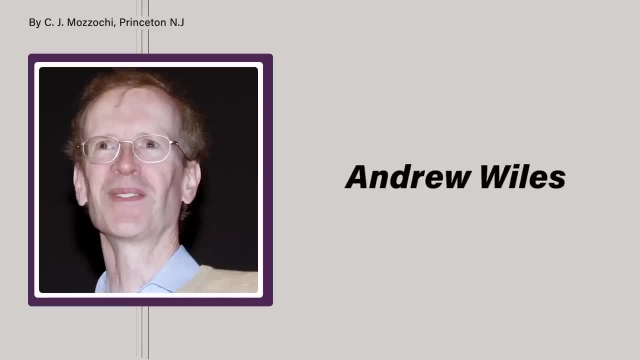 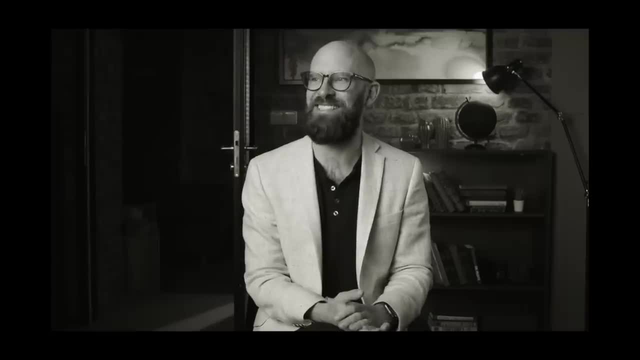 Andrew White. The problem was finally solved by British mathematician Andrew White. The problem was finally solved by British mathematician Andrew White. The problem was finally solved by British mathematician Andrew White. The paradoxes do not end at our innate ability, or lack thereof, to understand. 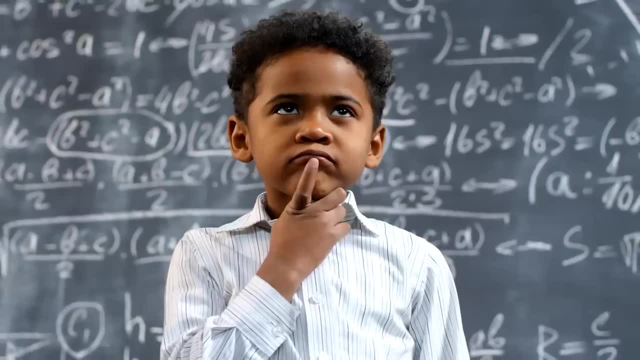 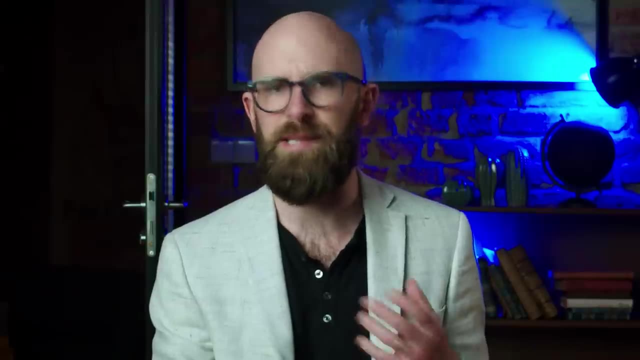 maths. They also extend to our desire to do it Among students from kindergarten all the way through high school. maths routinely polls as the least popular subject in school. However, when those exact same students are asked what their favourite subject in school is, one's 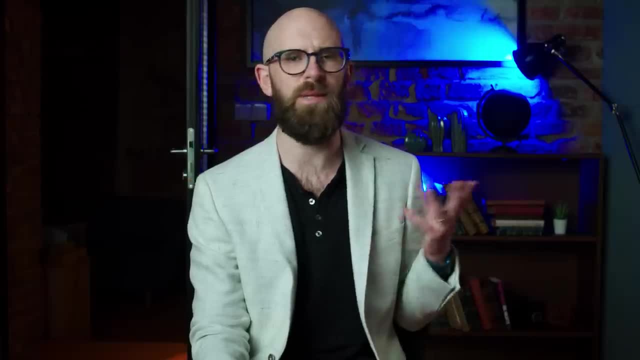 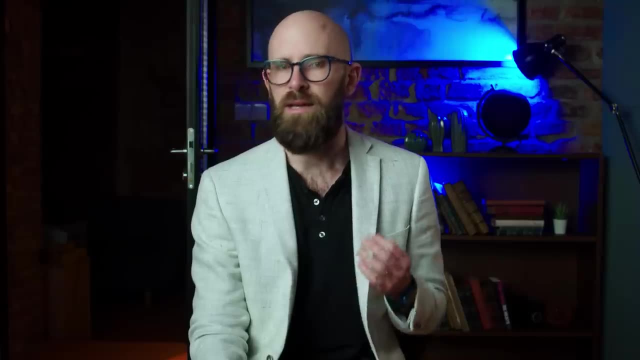 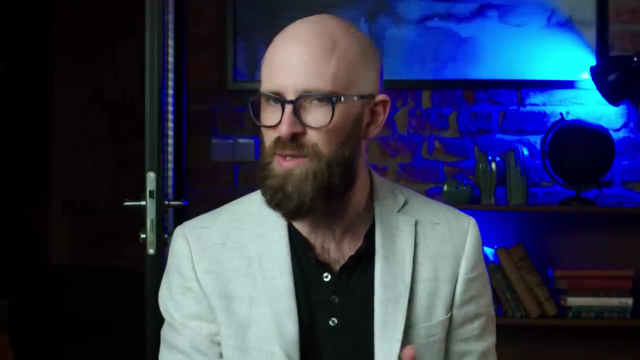 again, math does top the charts. it's simultaneously both the most loved and most hated subject by school children. but perhaps more students would take an interest in maths if they understood what was at stake. not only can mathematicians command much higher salaries than the median income, there are huge rewards in play as well for his seven years of hard work on format's last theorem. 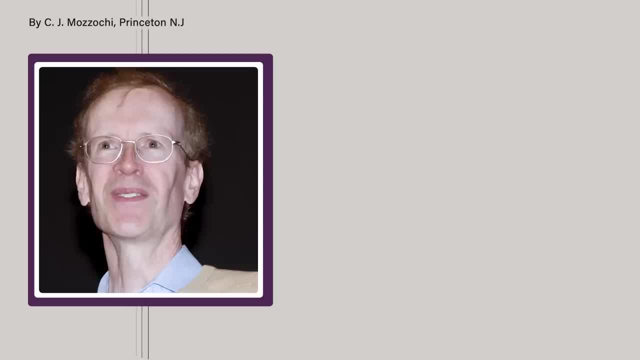 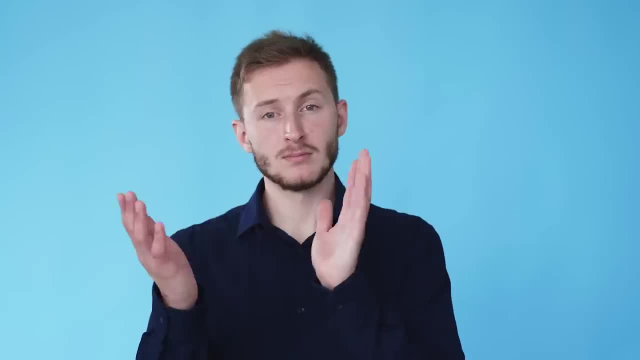 what exactly does andrew wiles have to show for it? well, for starters, you can address him now as sir andrew wiles, as his accomplishments was important enough to get him knighted by the queen. but if accolades don't do it for you, how about some cold hard cash money following his proof? 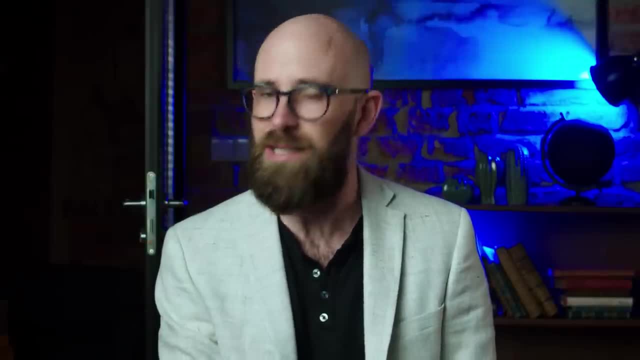 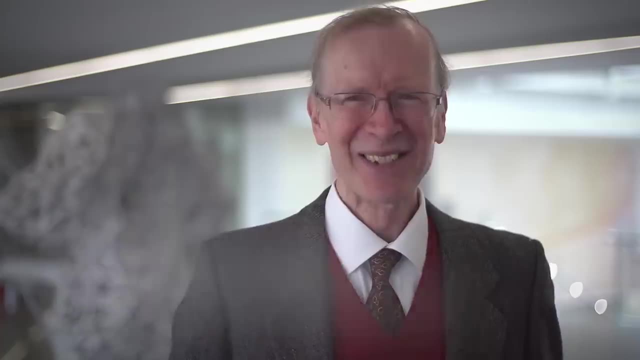 wiles received a mccarth fellowship, colloquially known as a genius grant. it's a five hundred thousand dollar grant given to individuals as an investment in their future, but with absolutely no strings attached. wiles was also given the able prize, an award for mathematicians awarded annually. 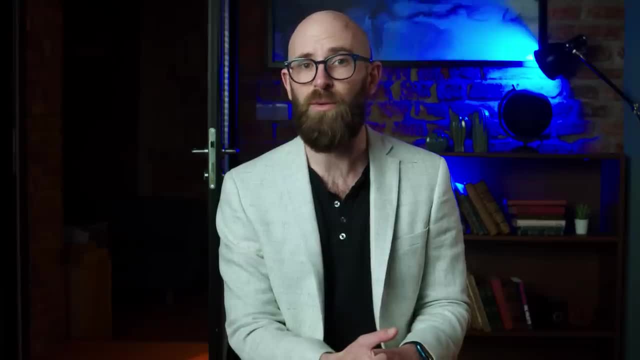 by the king of norway and it comes with 7.5 million norwegian kroner, which is approximately eight hundred and fifty million kroner, which is approximately eight hundred and fifty million million kroner, which is approximately eight hundred and fifty million kroner, which is approximately. 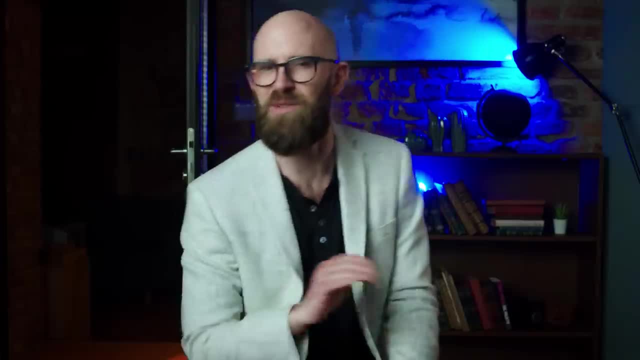 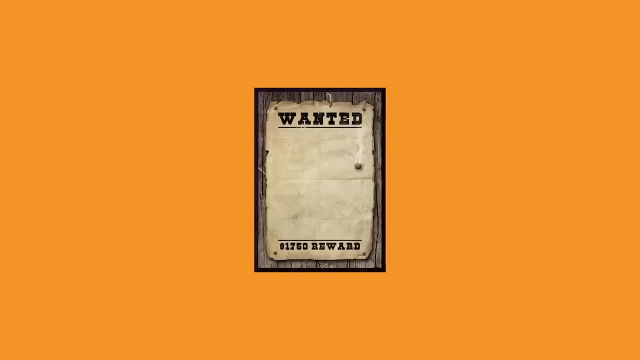 eight hundred and fifty million kroner, which is approximately eight hundred and fifty million thousand dollars. for those not willing to roll the dice that their mathematical discoveries will be important enough to earn one of these large cash rewards, there is some good news. there are a number of specific maths problems for which there is a cash bounty given to the first person. 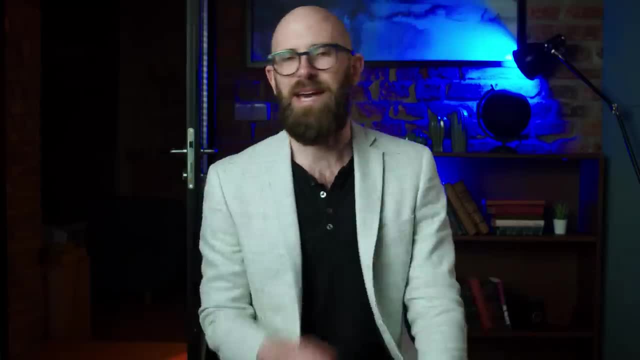 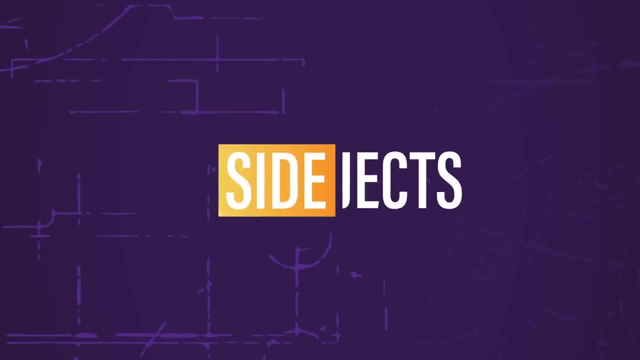 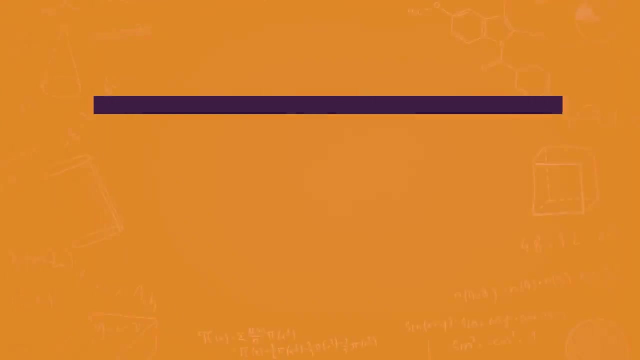 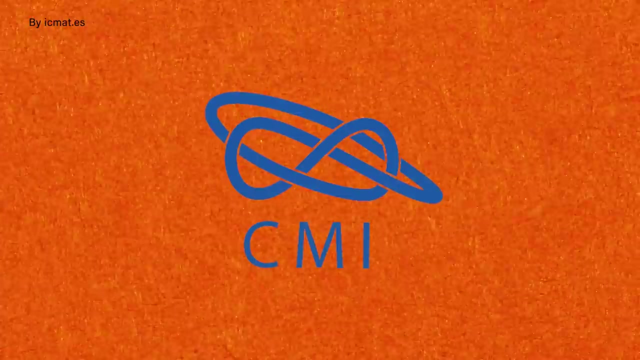 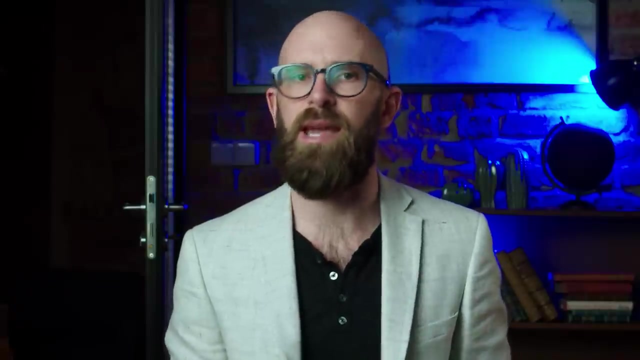 to solve them. the most famous of these are the millennium prize problems, a set of seven maths problems worth one million dollars each. the clay mathematics institute, or cmi, was founded in 1998 by businessman landon t clay. it's a private, non-profit organization dedicated to the study and dissemination of mathematical knowledge in 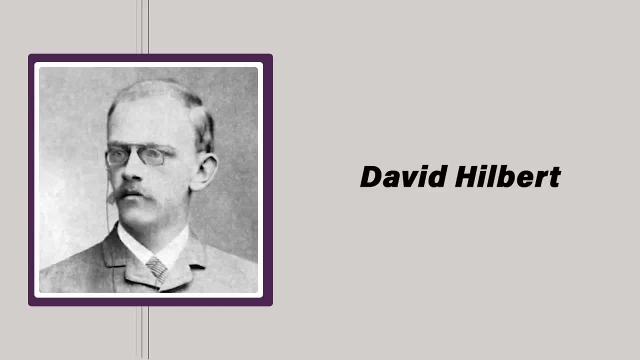 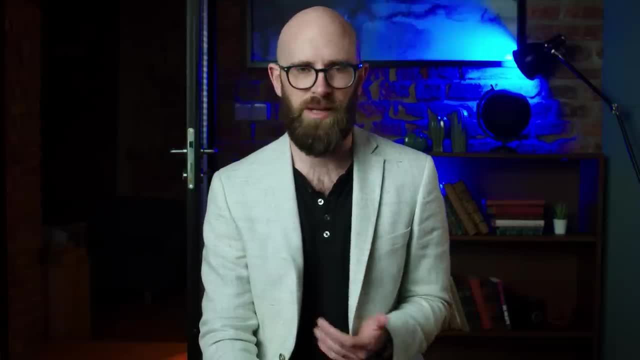 1900, german mathematician david hilbert published a list of 23 maths problems that were unsolved at the time. these problems, most of which are now solved, were extremely influential for the developments of mathematics in the 20th century. There were two problems with his list, however. 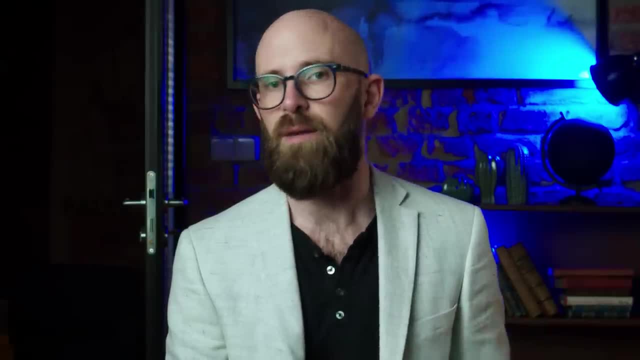 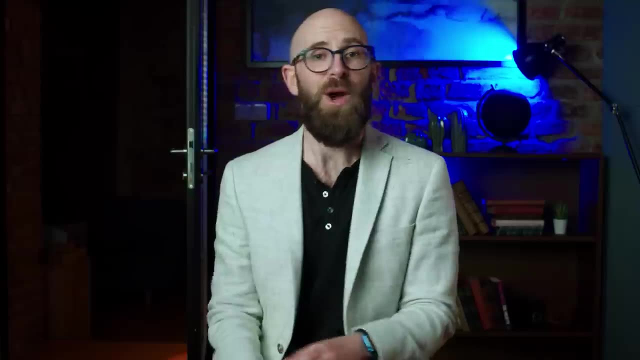 The first is that some of the questions were overly vague, meaning that there was no way to reach a consensus on whether or not the problem had been solved. The second was that the only prize for solving these problems was Hilbert's admiration. Drawing on Hilbert's problems as inspiration, CMI released its own list, the Millennium. 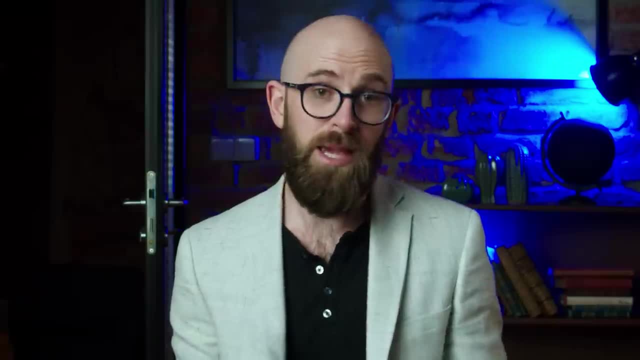 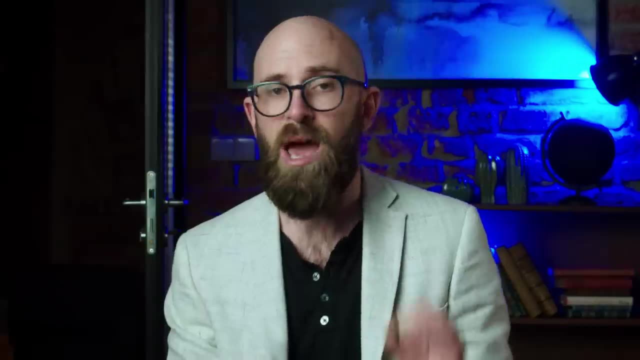 Prize Problems on May 24, 2000.. To combat the issue of vagueness that plagued some of Hilbert's problems, each of the seven problems has an official statement written by a professional mathematician, providing a very clear guideline for what each solution must entail. 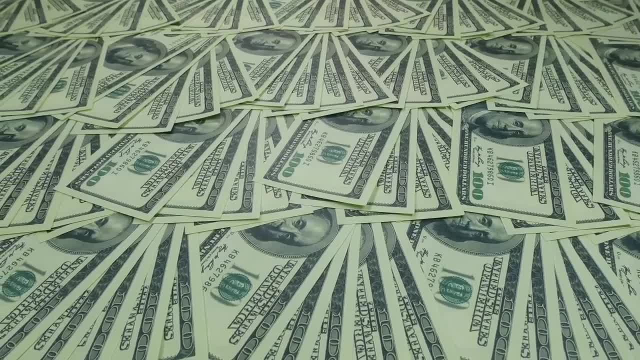 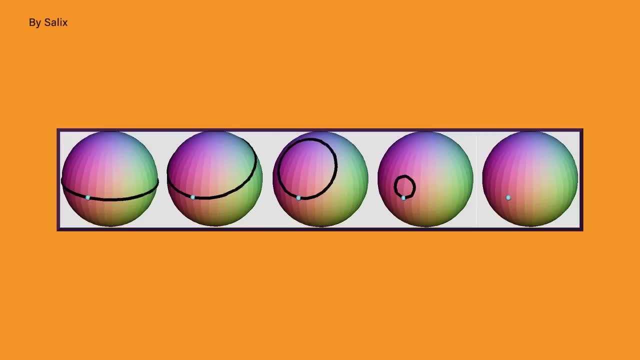 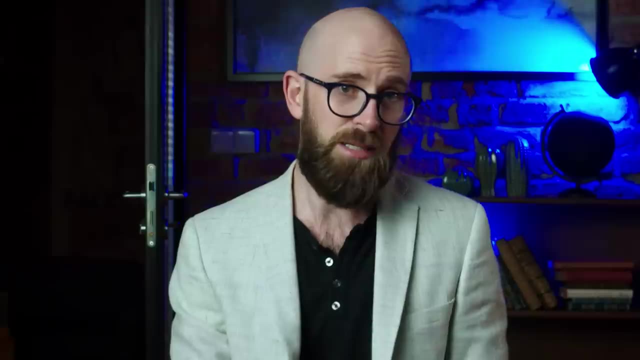 CMI also offered a monetary prize of a million dollars to the first person to solve each of the problems, which is certainly more appealing than admiration. To date, only one of the seven problems has been solved, meaning there is still six million dollars up for grabs for anyone with the talent and dedication to tackle these problems. 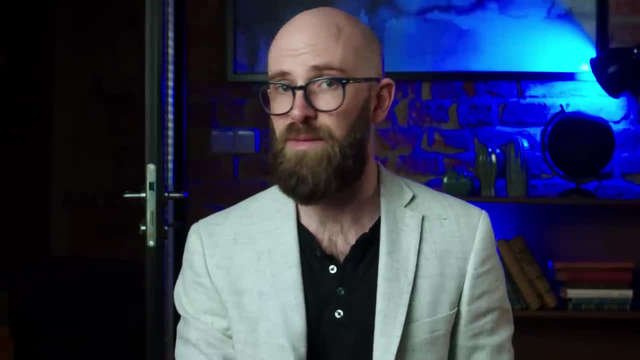 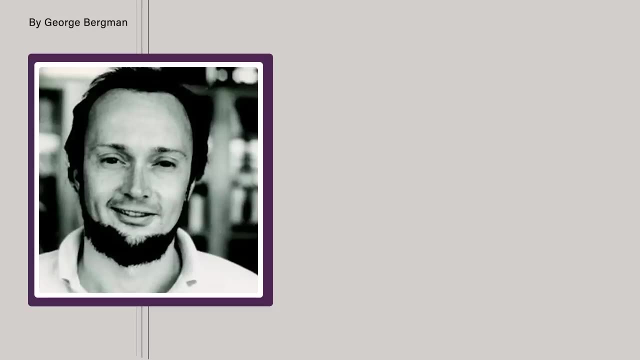 Despite one of the problems being solved, no prize money has been paid. This isn't because the CMI isn't true to their word, but rather because Russian mathematician Grigory Barman declined the prize. He felt the prize should have been offered to American Richard S Hamilton, as well as 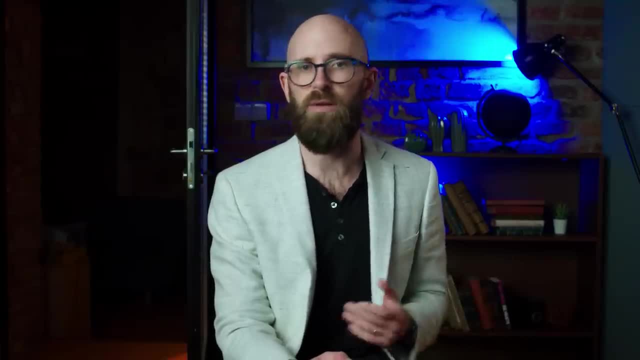 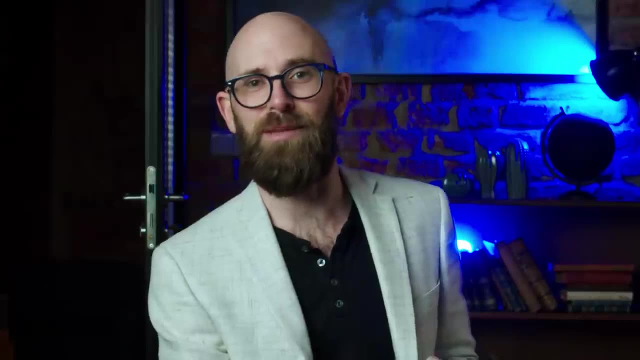 it was Hamilton's work that Perelman built the solution on top of, and apparently Perelman's integrity is worth more than a million dollars. Good for you, mate. This was the fourth award for mathematics that Perelman had won, and the third that 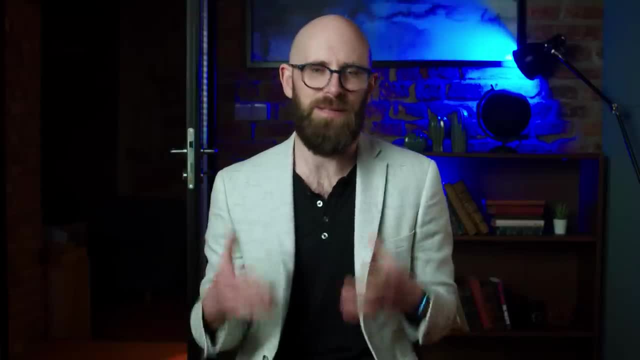 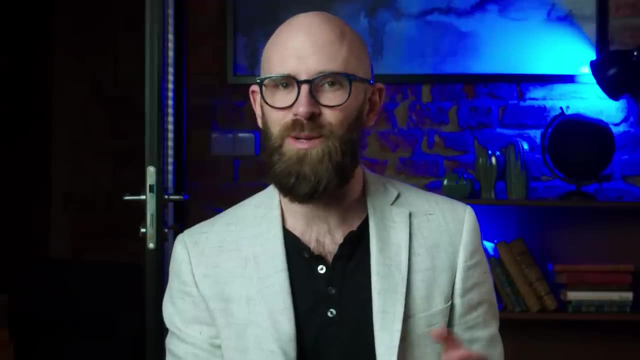 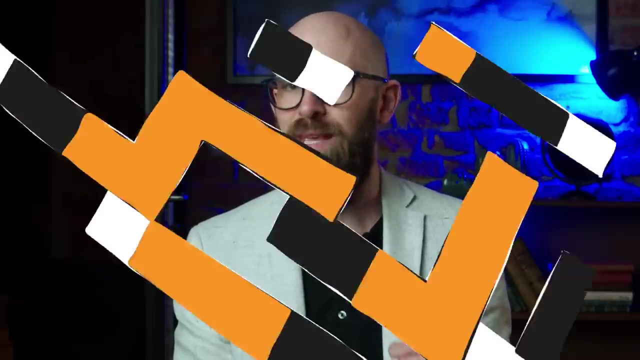 he declined. At this point you may be wondering what exactly these problems are. Some of them are far too complex for the scope of this video, Not a good sign for anyone with only a casual interest in becoming a maths-based millionaire. but we'll examine the ones that we can. 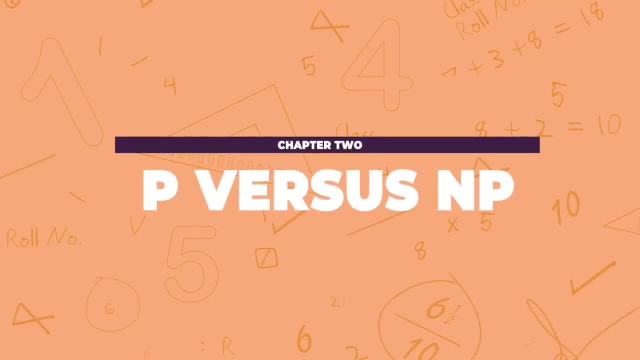 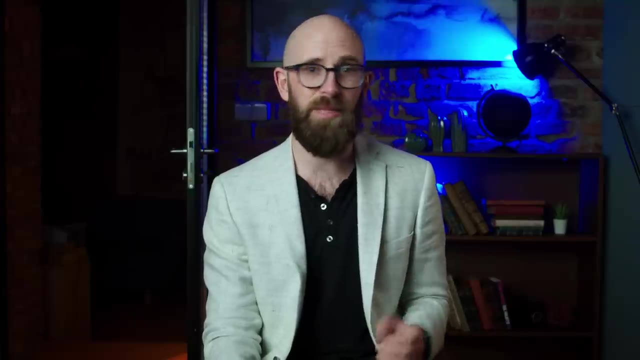 The B vs MB Problem. The B vs MB problem is a major unsolved problem in computer science. It is a particularly frustrating problem because, like Fermat's Last Theorem, the vast majority of mathematicians and computer scientists agree on what the solution is. 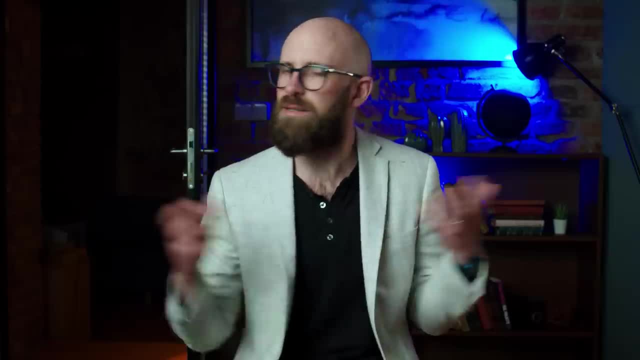 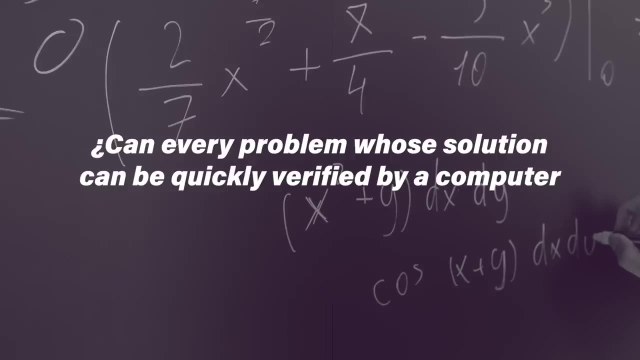 The problem is that the problem is not solved. They just don't have a way to prove it. The fundamental question of P vs NP asks: can every problem whose solution can be quickly verified by a computer also be quickly solved by a computer? 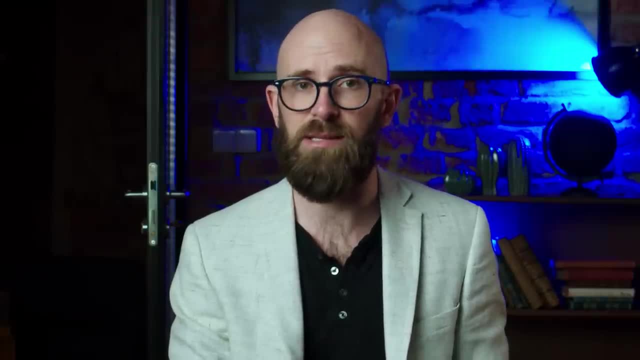 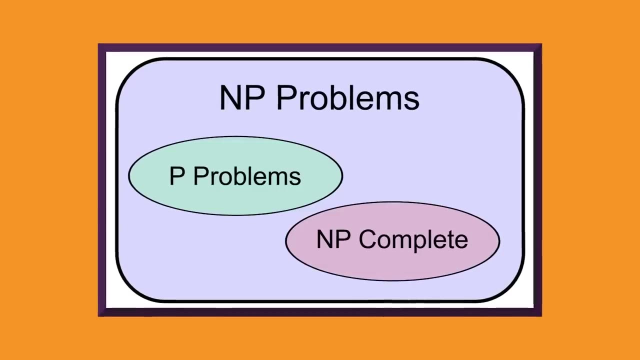 As of 2019,. it was believed by 99% of experts that the answer to this question is no. The problem creates two sets of algorithms: P and NP. P stands for polynomial time and NP stands for non-deterministic polynomial time. 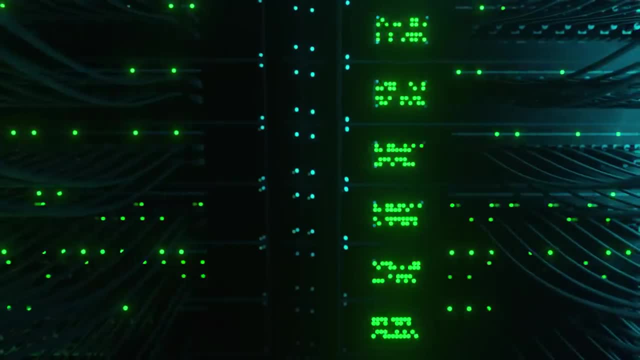 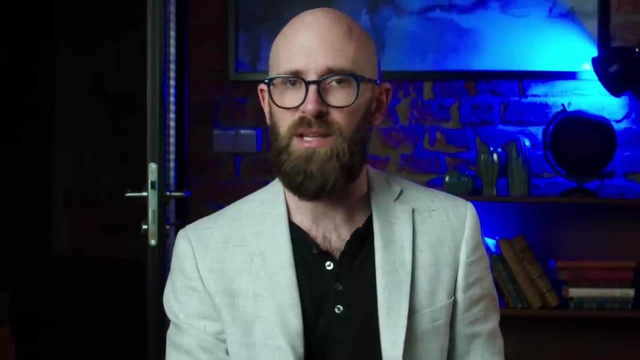 Polynominal time is a specific algorithm used to gauge how long it takes for a computer to complete a task. The simple version is that something in polynomial time is fast and something not in polynomial time is slow and thus unfeasible from a computational standpoint. 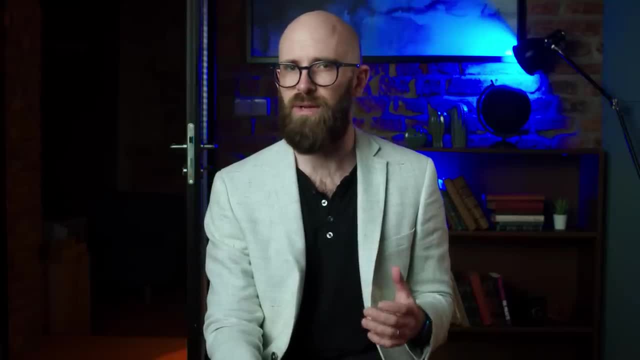 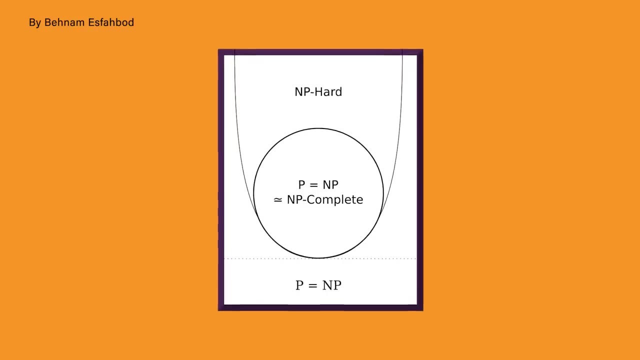 In this problem. P represents all questions that an algorithm can find an answer to quickly. NP represents all questions that an algorithm can verify an answer to quickly. The problem is: does P equal NP? Can every question that can be quickly solved by a computer also be quickly solved by a? 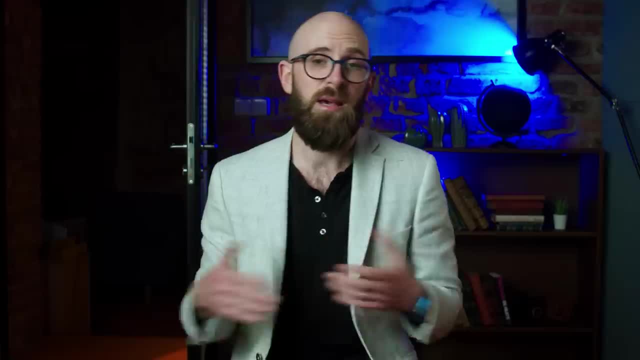 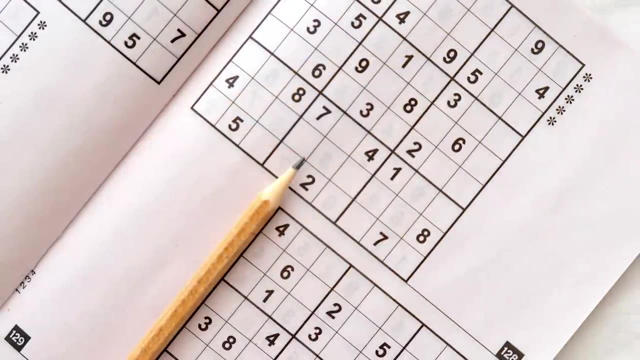 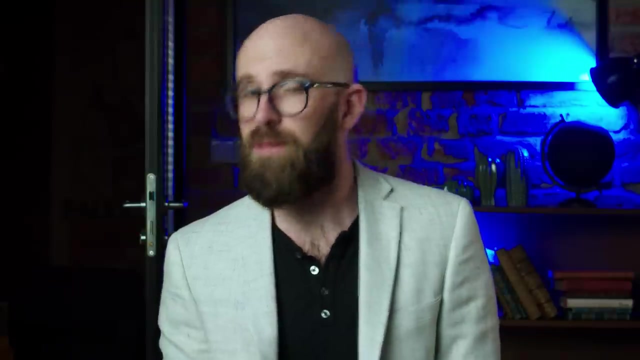 computer quickly verified also be quickly solved? and again, the answer's probably not. for a more concrete example, thank you, kevin. let's look at a game of sudoku. the best solvers in the world can tackle even the hardest classical sudoku puzzles in a matter of minutes. so naturally a computer algorithm. 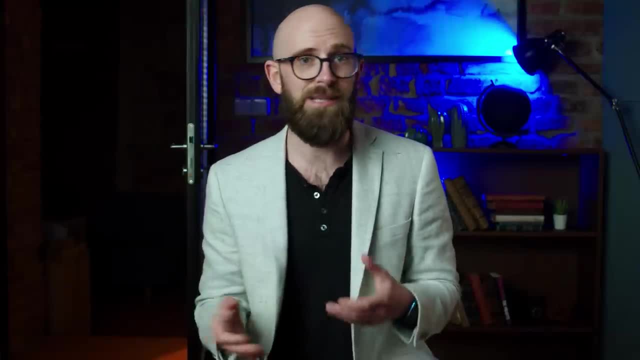 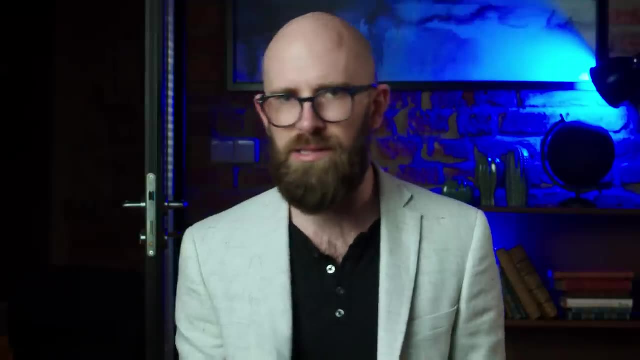 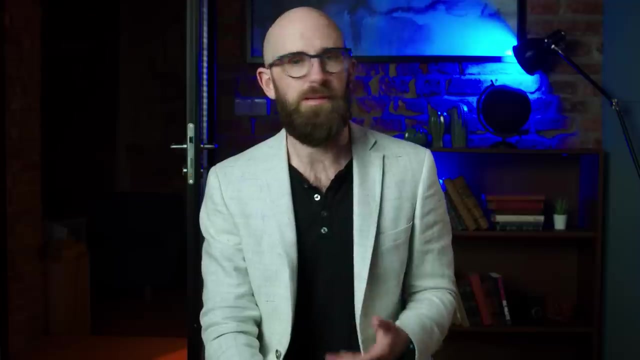 can do it even faster. likewise, verifying that a completed sudoku is correct takes under a second for a computer. however, what happens if the grid becomes larger? while a nominal 9x9 sudoku could be quickly solved by an algorithm, the same can't be said for a 100 by 100 sudoku. the time to verify. 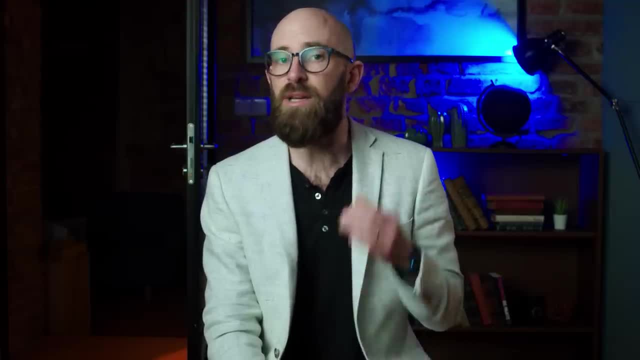 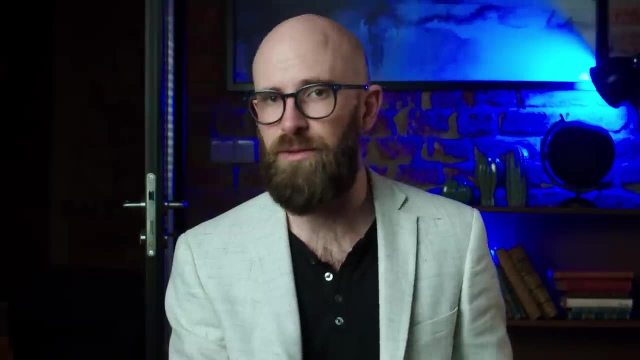 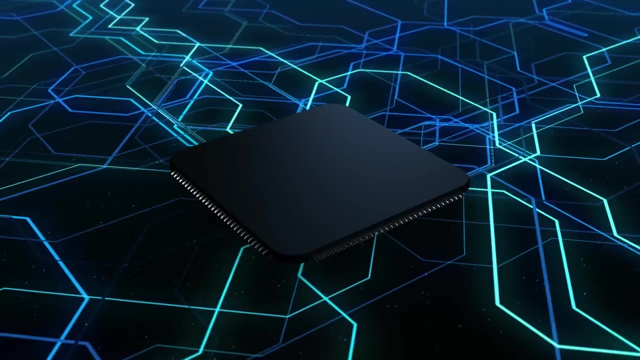 the solution increases linearly with complexity, but the time to solve one increases exponentially. verifying that the 100 by 100 sudoku contains each number 1 through 100 exactly once in each row, column and box is trivial, but actually solving such a problem is a herculean feat, even for a 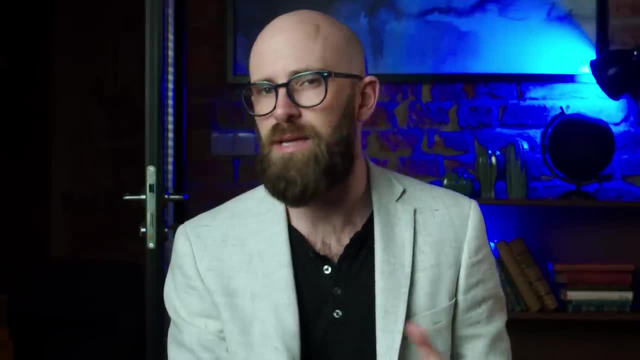 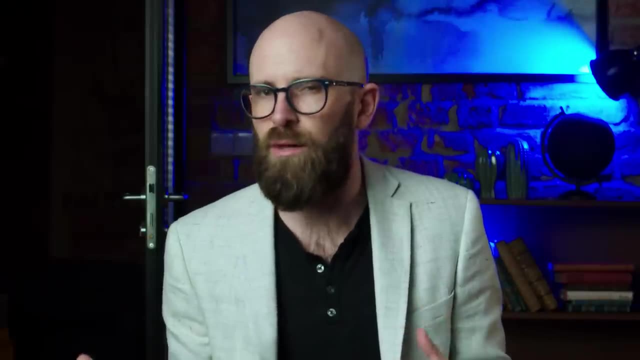 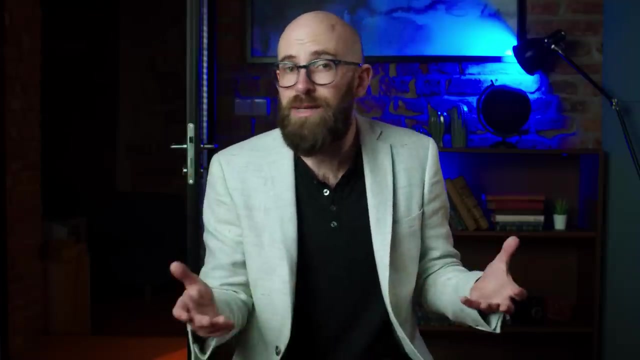 computer. so that's it, then. we've just proved that p does not equal np, because we know of problems that can be quickly verified but not quickly solved, right? well, no, we haven't actually proved that it is impossible to solve such a problem quickly, just that we don't currently know how to. for this reason, a contra proof is extraordinarily. 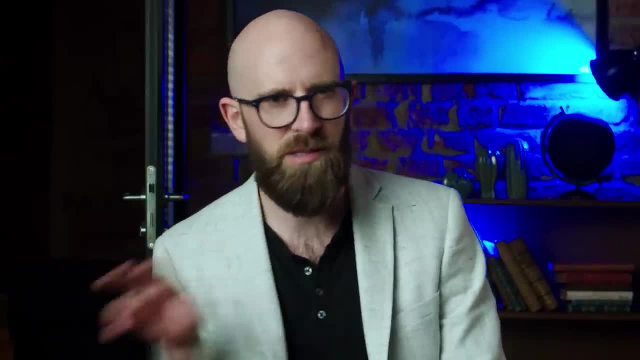 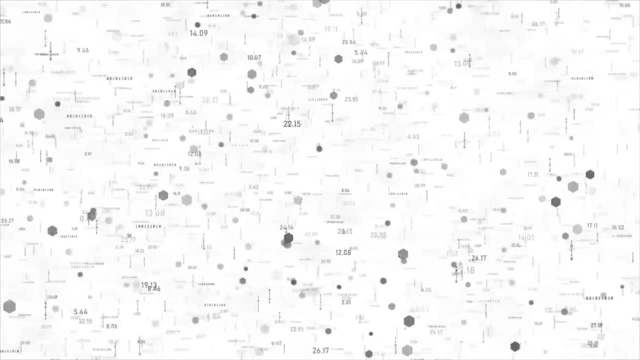 difficult, as a person would not just need to prove that we are unable to solve such a problem quickly, but that, even with all the knowledge in the universe, doing so would be fundamentally impossible. i get it, i get it. do you get it? i get it, i did get it with all the math talk and i'm like hey. 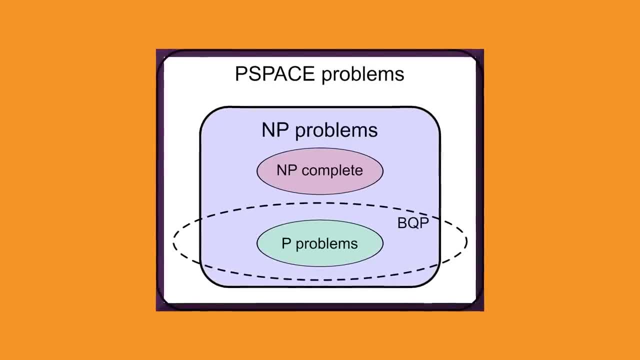 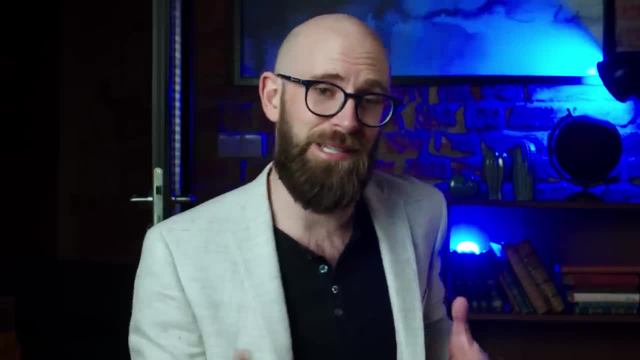 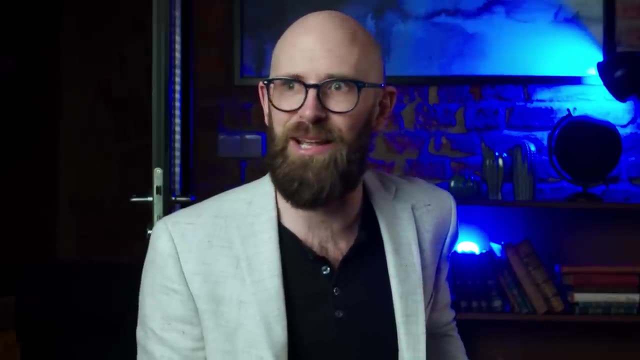 p versus mv is an important problem in computational complexity theory and an answer to the problem would be invaluable, more importantly, if someone could prove the experts wrong and somehow show that in fact p does equal mp. the implications for future computing technology are absolutely massive. that yeah, of course. then it'd be like super computer being super smart. 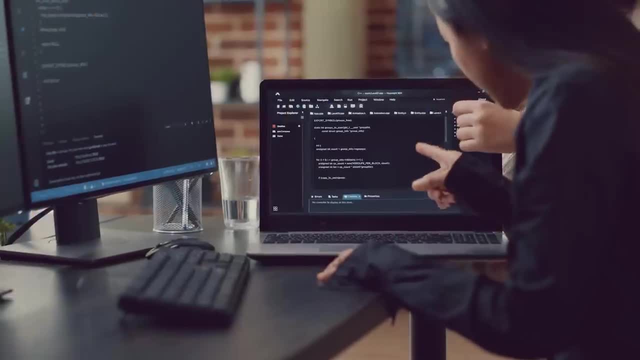 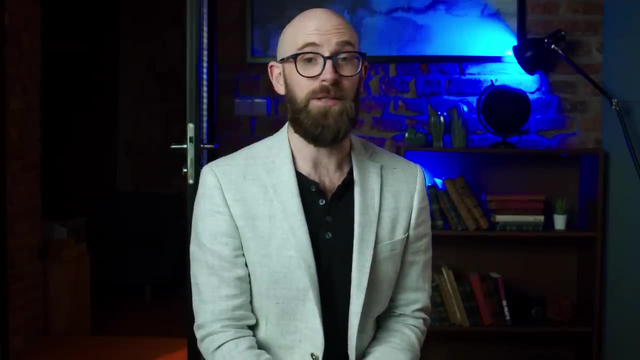 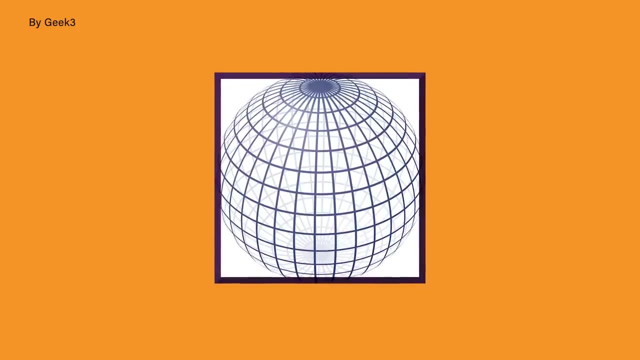 if complex computer algorithms aren't your thing, why not relax, crack open a beer and take some time to consider the physics behind the poor of your frothy beverage of choice? the navius stokes equations are a system of differential equations that describe the motion of fluid in 3d space. they 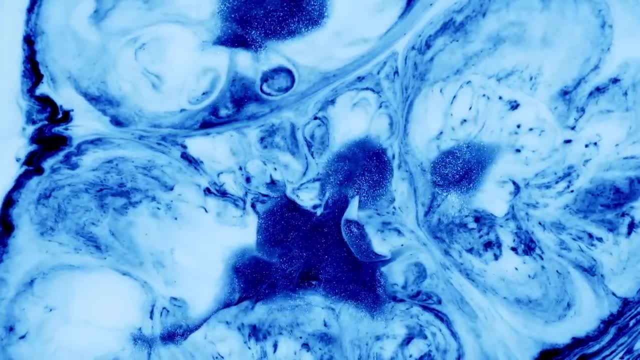 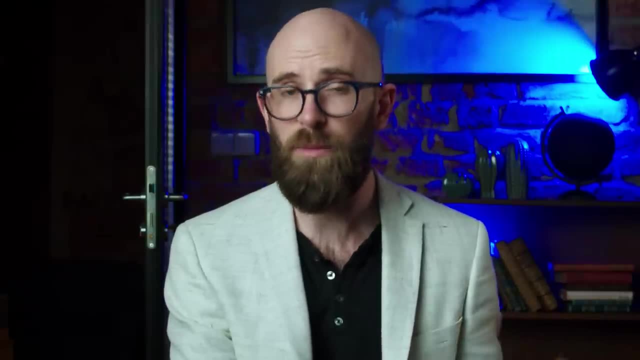 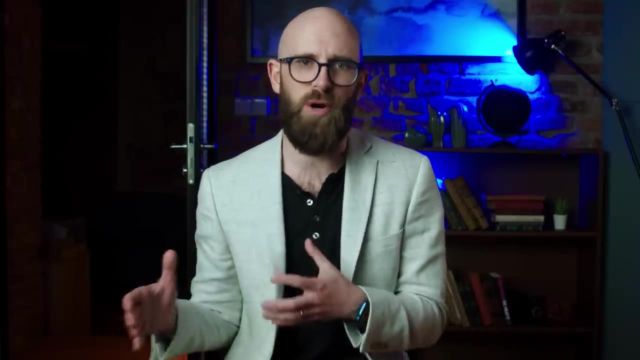 are fundamental to our understanding of fluid dynamics and are extremely important in science and engineering. they're an important set of equations with a wide range of practical applications and are commonly in use today. the only problem is that the equations aren't complete. even some of the most basic and intuitive properties of the solutions to navier-stokes equations have not. 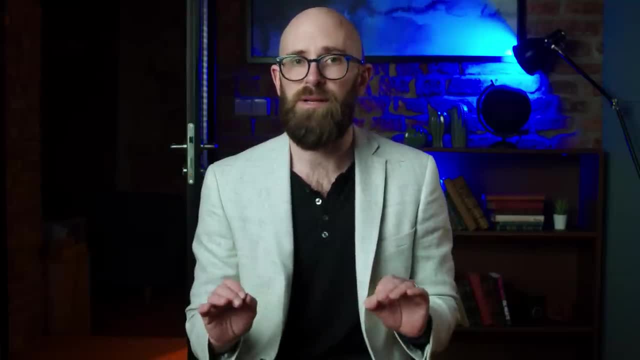 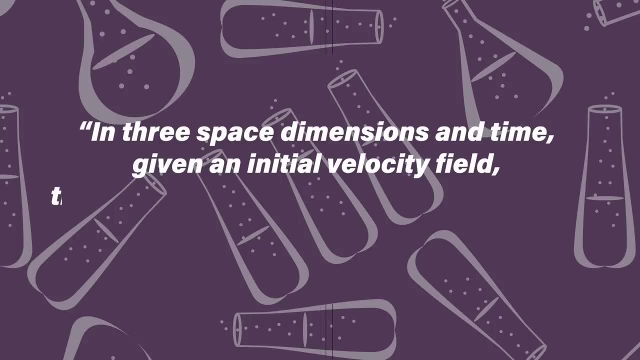 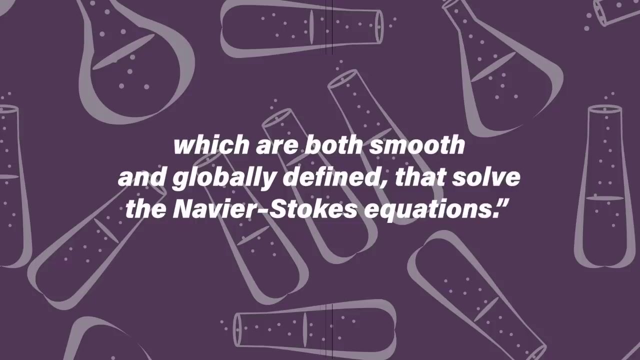 actually been proven. the official statements of this millennium problem reads as follows: prove or give a counter example of the following statement: in three space dimensions in time, given an initial velocity field, there exists a vector velocity and a scalar pressure field which are both smooth and globally defined. that solve the navier-stokes equation. 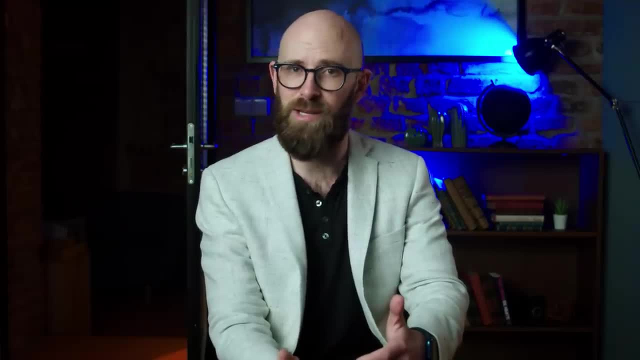 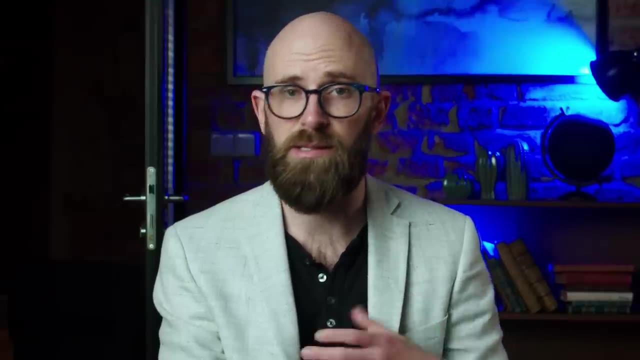 essentially, they're asking to either prove that the navier-stokes equations are always true or show an example where they're not smooth and globally defined. basically means that the equations are consistent and universally applicable. this to even be a question. that means that, despite being heavily 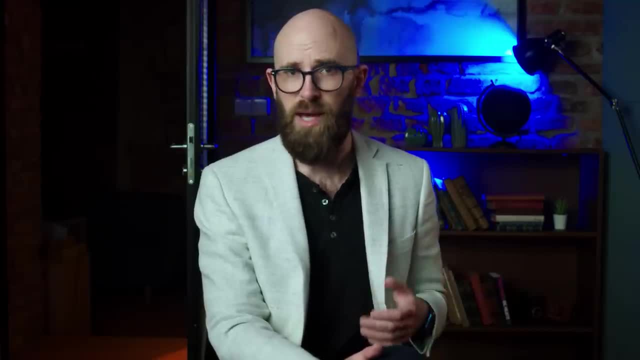 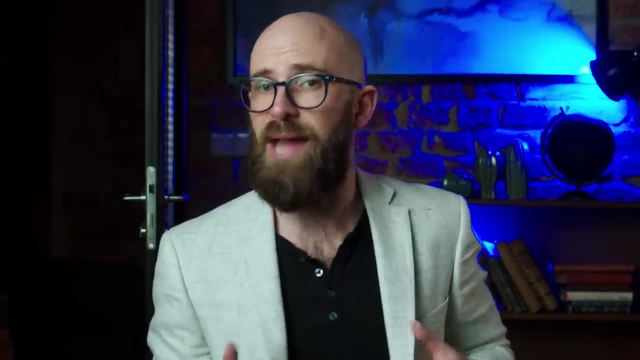 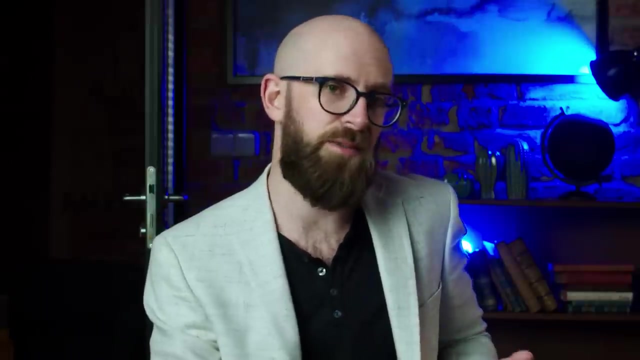 used in science and engineering. a counter example has yet to be found. so, in fact, the navier-stokes equations have already been proven in limited capacities. when only dealing in two-dimensional space, there are smooth and globally defined solutions. likewise, when the initial velocity is small enough, these solutions do also exist in 3d space. to discover an answer under unrestrained 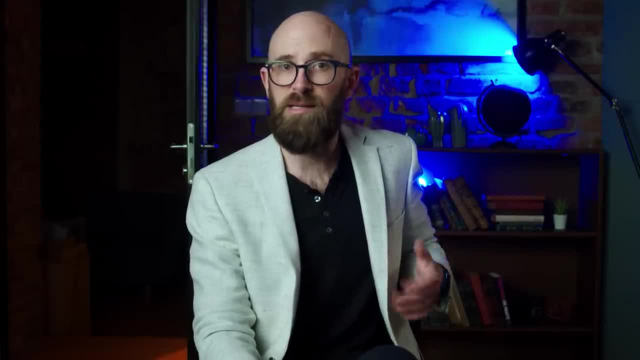 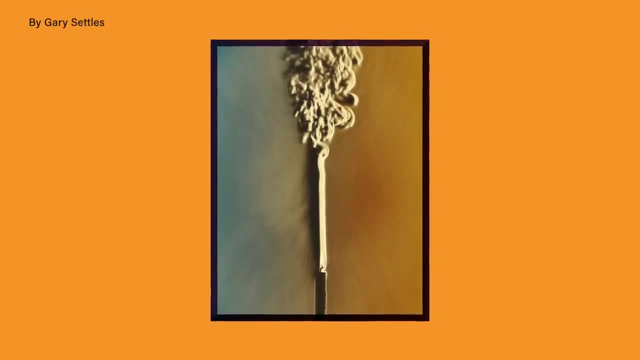 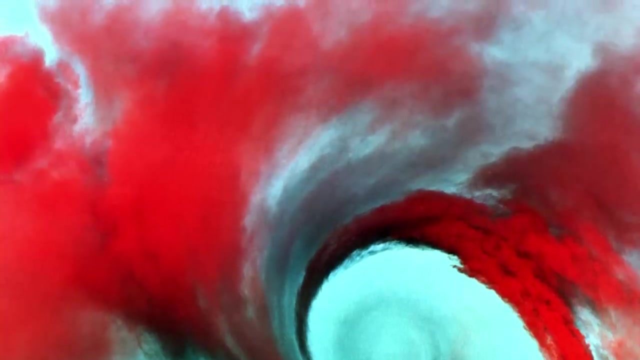 initial conditions, however, would be a giant step in understanding one of physics's oldest questions: what the is turbulence in fluid dynamics? turbulence is seemingly chaotic changes in pressure and flow velocity. that's about all we know about it. fully solving the navier-stokes equations could give us a greater understanding of turbulence in fluid and, ideally, lead to a 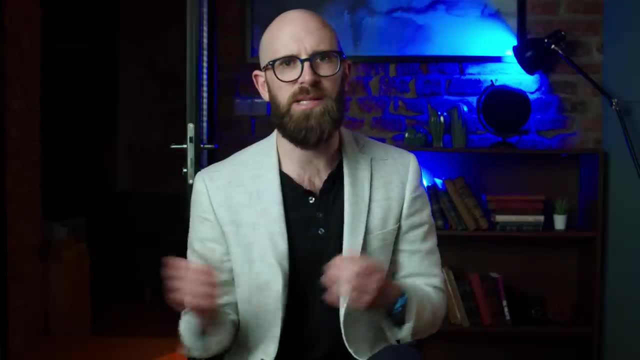 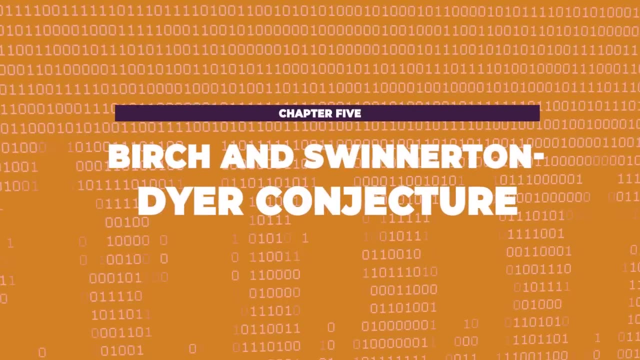 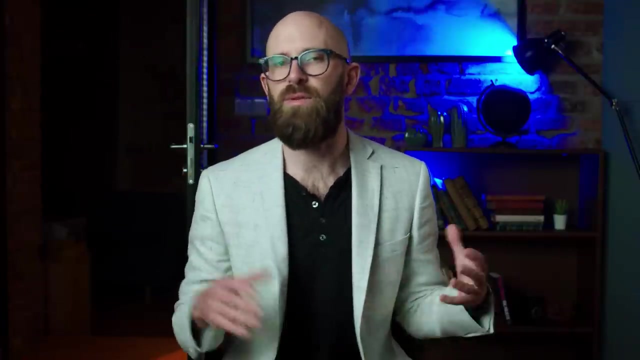 theoretical model to describe how turbulent flow works without using scientifically vague terms like chaotic. the birch and swinner's entire conjecture deals with equations that define elliptical curves over the rational numbers. rational numbers are every number that can be written as a ratio like 5 over. 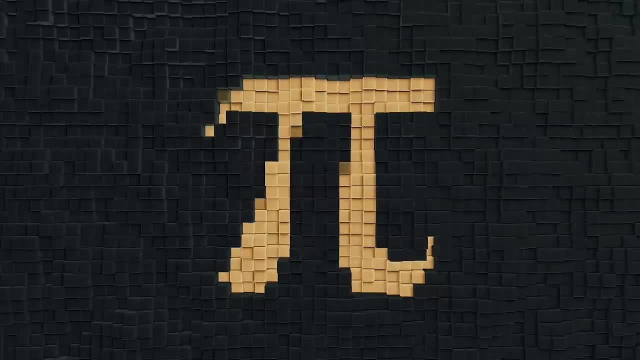 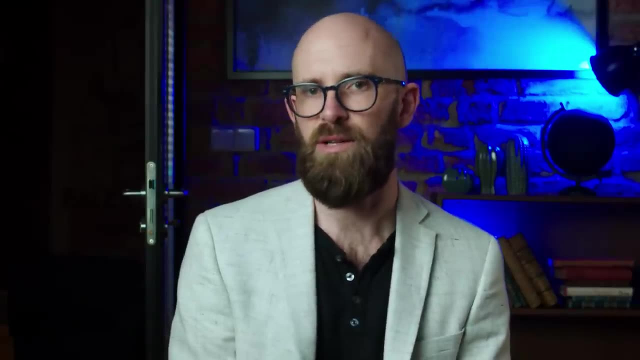 19 or 8 over 1.. so it excludes numbers like pi, e and the square root of 2.. the conjecture is that there is a simple way to solve turbulence in fluid dynamics, and that's by using the navier-stokes to tell whether one such equation has a finite or an infinite number of rational solutions. that 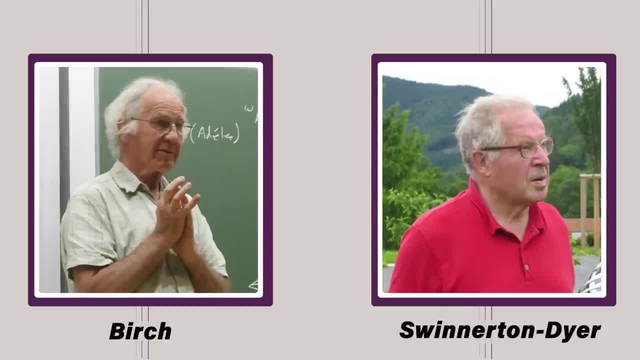 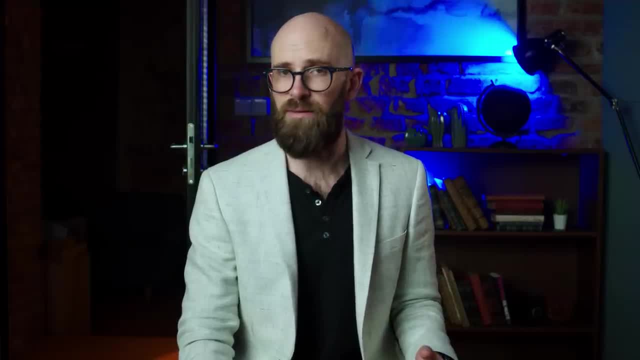 seems simple enough. the two mathematicians posited that there is an easy way to look at an equation and know whether or not it has infinite solutions. not only is it not simple- otherwise it wouldn't be one of the millennium problems- but it is regarded as one of the most complex problems in all of 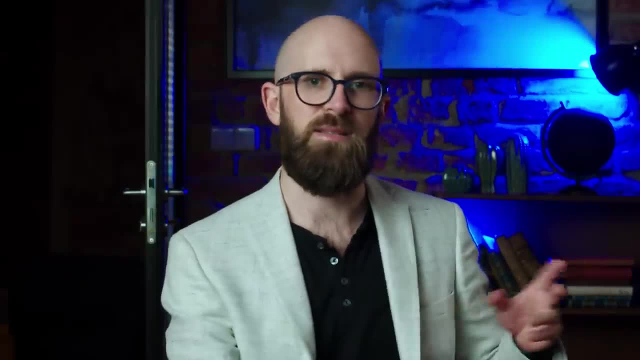 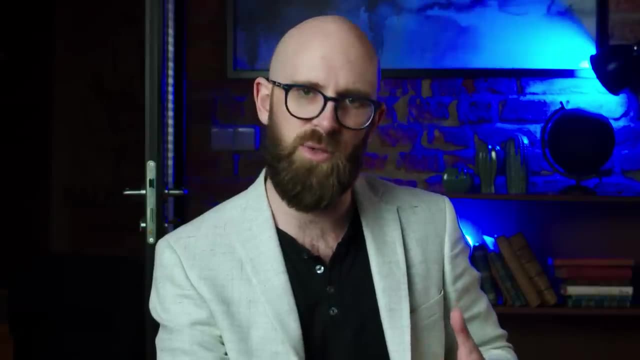 mathematics. the ruler was first proposed in the 1960s with the help of machine computation. it was developed at trinity college in cambridge, england, by two mathematicians, both of whom had the school. the conjecture was initially met with skepticism by birch's phd advisor, though evidence 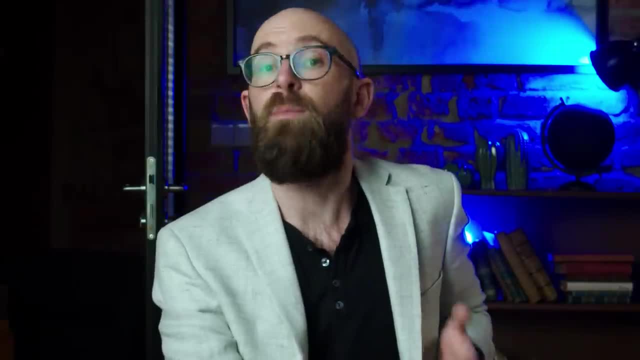 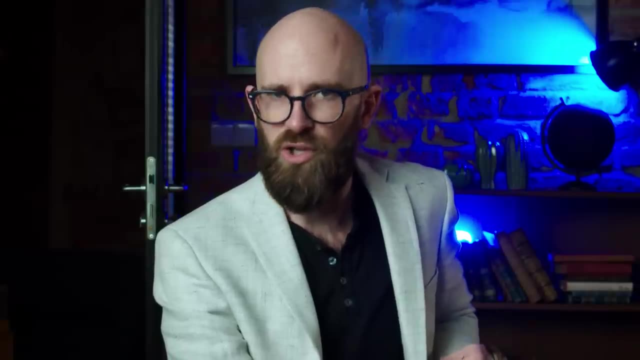 quickly began piling up. of course, evidence in maths is not proof. even with billions of pieces of supporting evidence, all it takes is a single counter example to show that a theory or conjecture is false, and with infinite numbers and equations, it is impossible to brute force a positive proof. 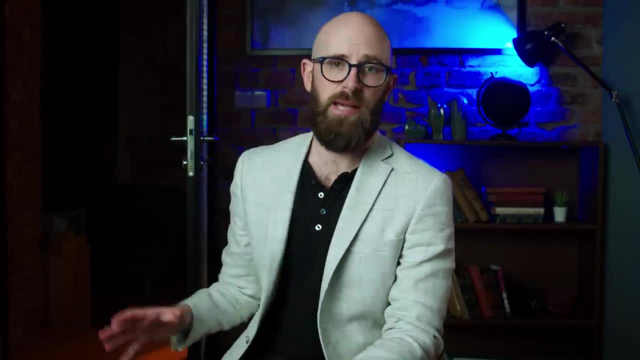 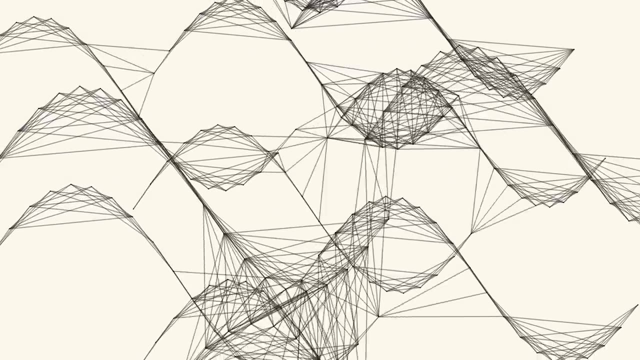 while the conjecture has not been universally proven, it is no longer the case that there is nothing definitive. starting in the 1970s, the conjecture began being proven for certain special cases. the original proofs only applied to modular elliptical curbs, though. in 2001 it was proven that all elliptical curves over rational numbers are modular, which extended 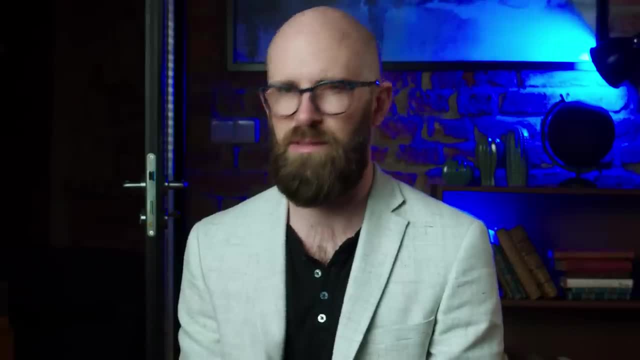 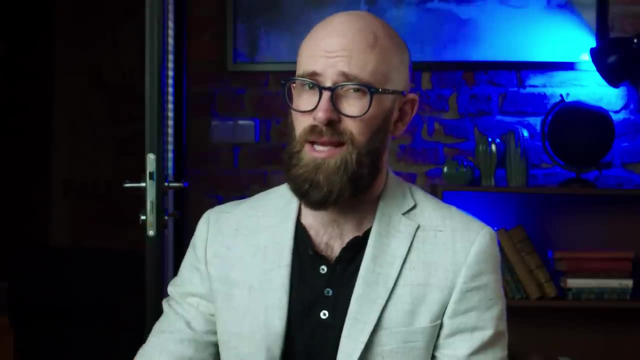 the utility of the existing proofs. however, all of the proofs thus far only handle curves with a rank of zero or one. there is extensive evidence for curves of higher rank, but thus far nothing has been conclusively proven. unfortunately, as multiple of the current special case proofs were made after 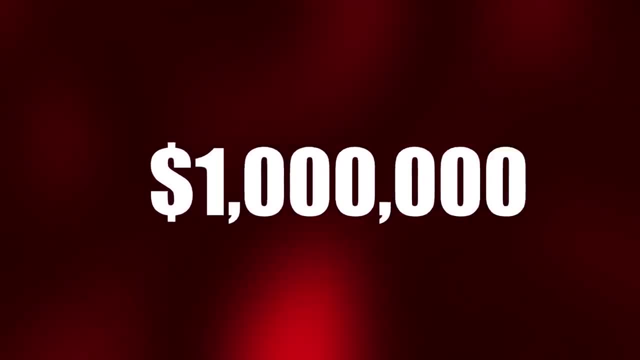 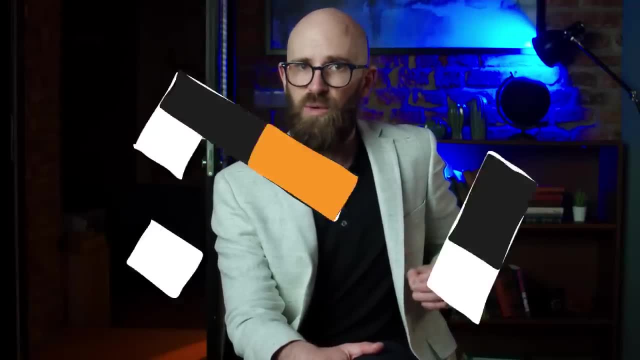 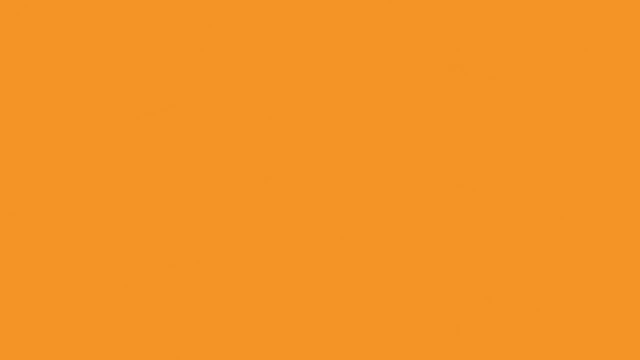 the year 2000. it is fair to say that cmi will not be handing over that one million dollars, unless you can devise a universal proof to the conjecture rather than just proofs for specific sets of elliptical curves. the rival hypothesis is named after german mathematician bernhard riemann, as 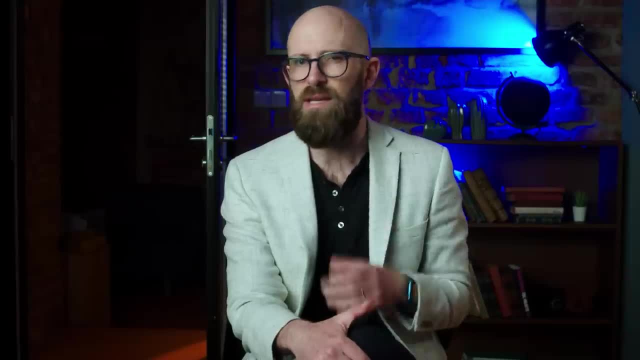 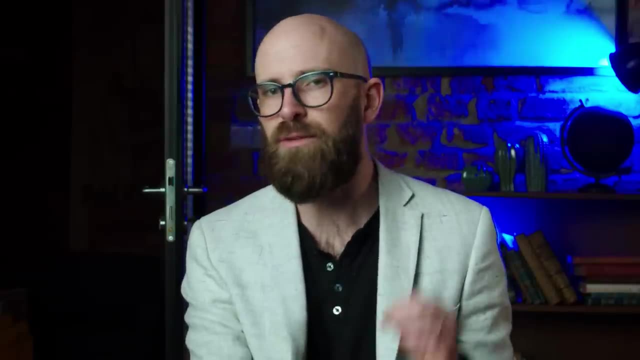 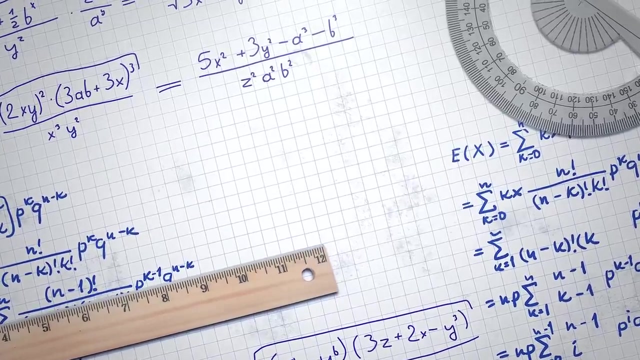 was originally proposed in 1859. it is considered to be the most important unsolved problem in all of mathematics, so important that it is the only one of hilbert's 23 problems that was reused for his puzzles. the ryman hypothesis is an interesting one for number theory, particularly because, if true, 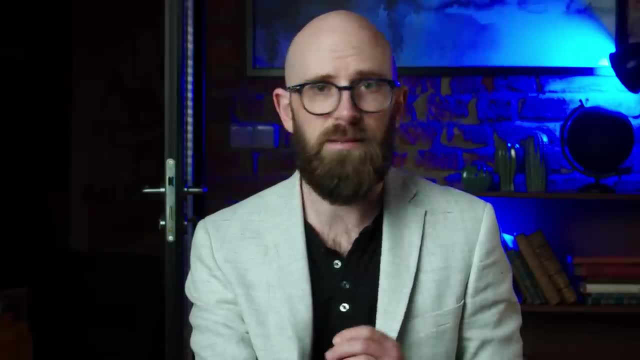 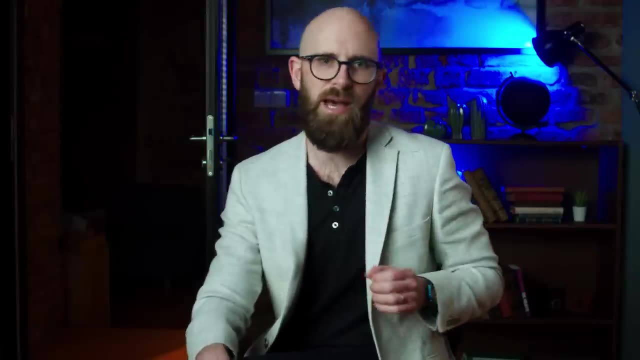 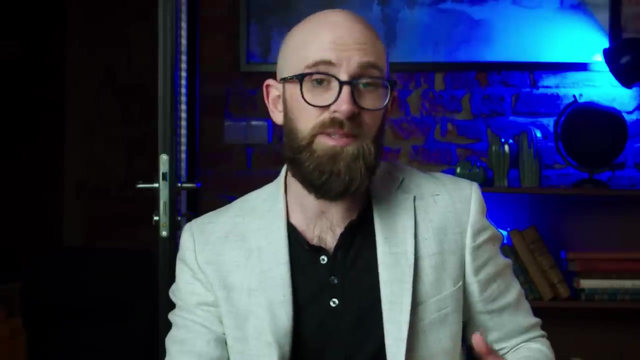 it implies results about the distribution of prime numbers, and there is nothing that gets mathematicians excited like discovering new prime numbers. aside from being a fun novelty, prime numbers do actually have a variety of practical applications, including their use in computer encryption methods. but just how difficult is the problem that has eluded the world's greatest? 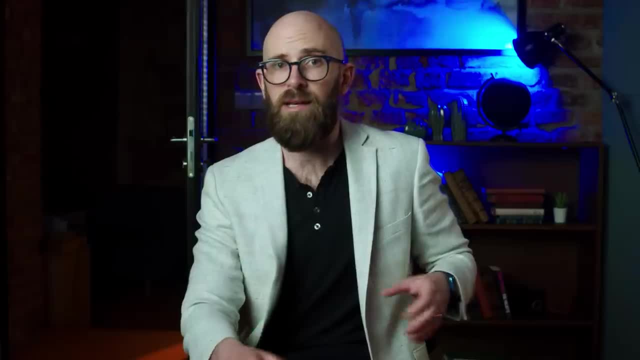 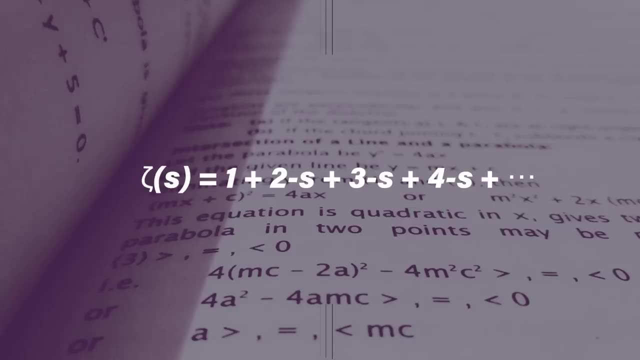 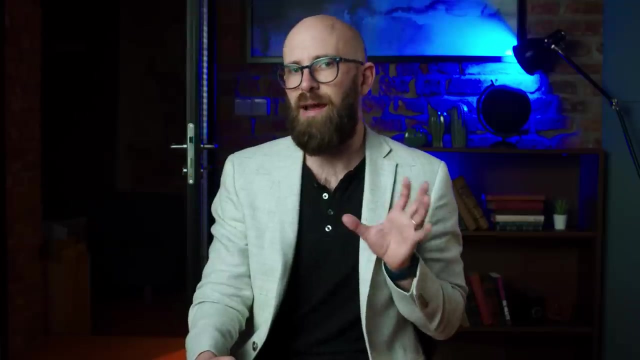 mathematicians for over a century. well, first consider the ryman's zeta function defined as well. let's just show it on the screen now. where s is any complex integer other than 1.. when s is a negative integer, minus 2, minus 4, minus six, etc. this function will have zero. 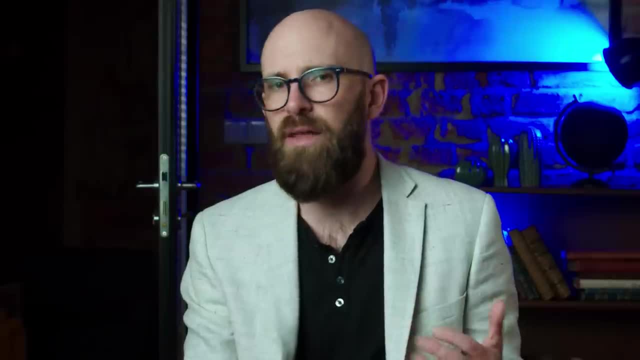 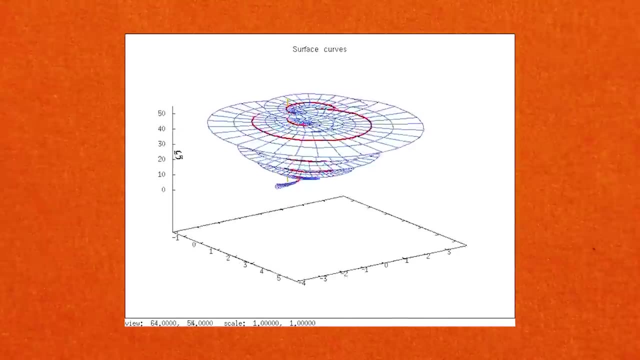 but these are called trivial zeros. however, there are other values of s that also have zeros, and these are non-trivial zeros and they are the ones that the hypothesis is concerned with. the hypothesis states that the real part of every non-trivial 0 of the ryman zeta function is half. 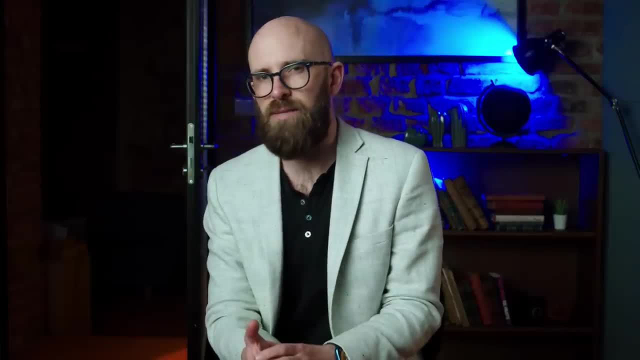 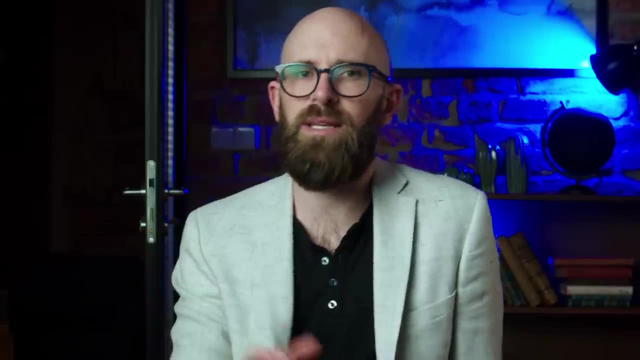 non-trivial zeros exist on the line of complex numbers defined as half plus i, t, where t is a real number and i is an imaginary unit. if that didn't make any sense to you, how did you know? kevin? even the people who did not understand every word about hypothesis are